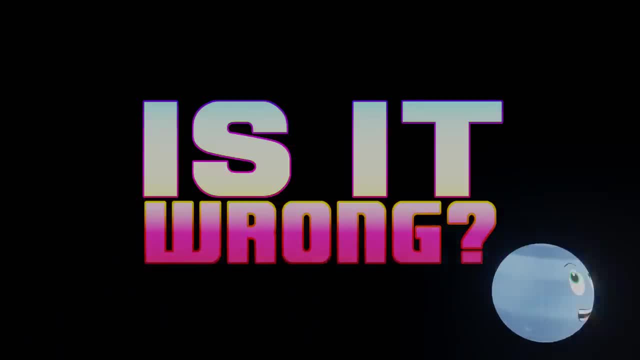 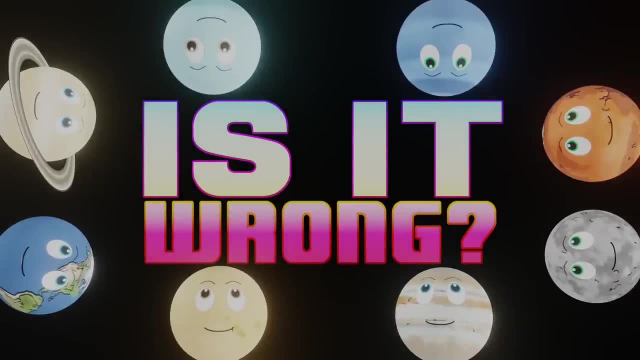 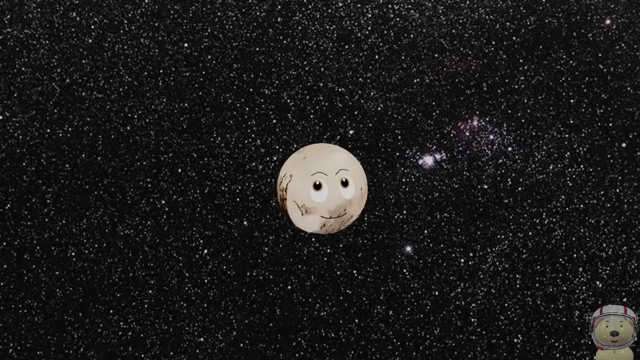 Is it wrong? Is it? Is it wrong? Is it wrong? now Tell me why you know it's wrong. Is it wrong? Is it Is it wrong? Dwarf planets have no moons. Some people think that dwarf planets have no moons. 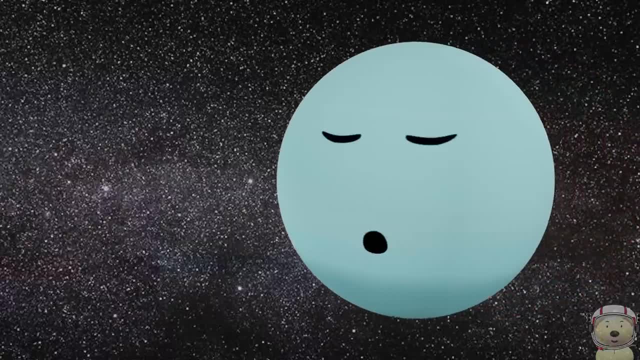 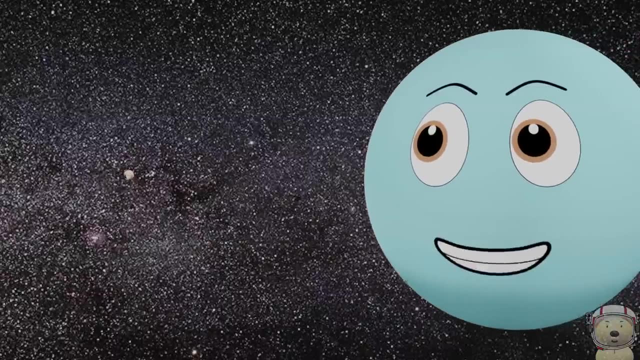 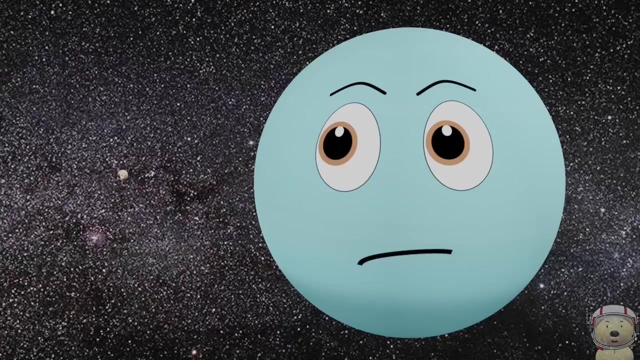 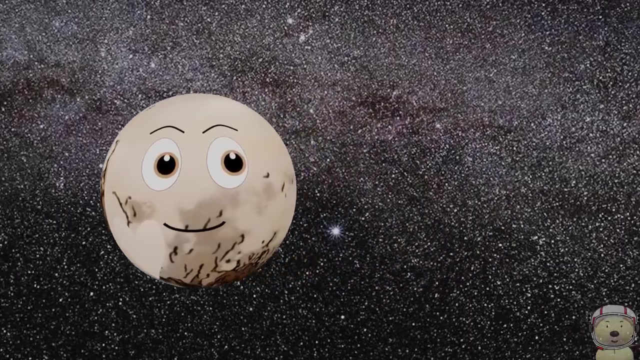 Wrong. Wait, wait, wait, Pluto. We have always said that you are Make way centre stage. centre stage, Not a planet, Ah, I know. So you can't have moons There, Not true Uranus? In fact, some of us dwarf planets have more than one moon. 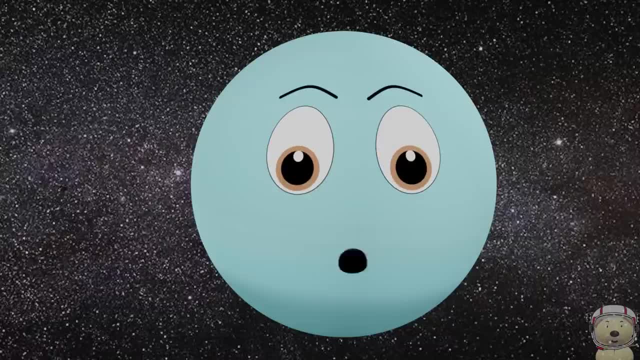 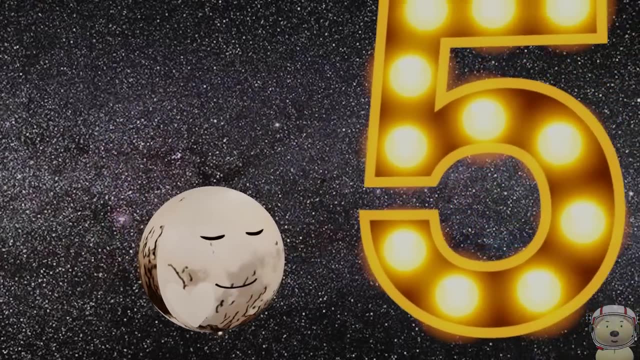 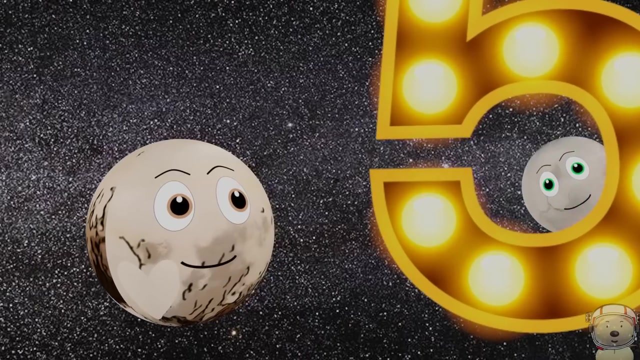 I'd like to see that. Well, actually I wouldn't. I'm off. I actually have five moons, one of which is half the size of me. Don't care, Here's Charon, my biggest moon. Look how big Charon is compared to me. 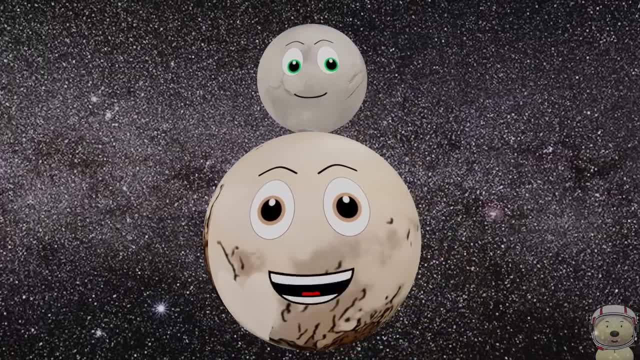 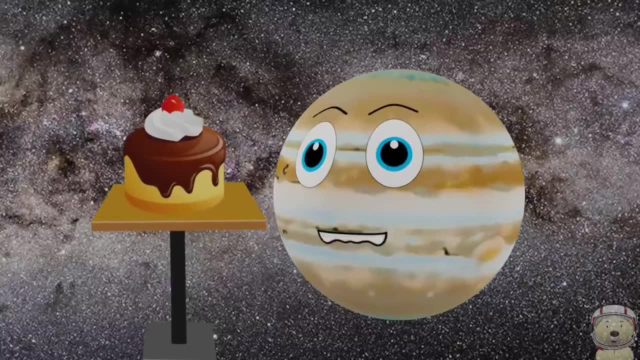 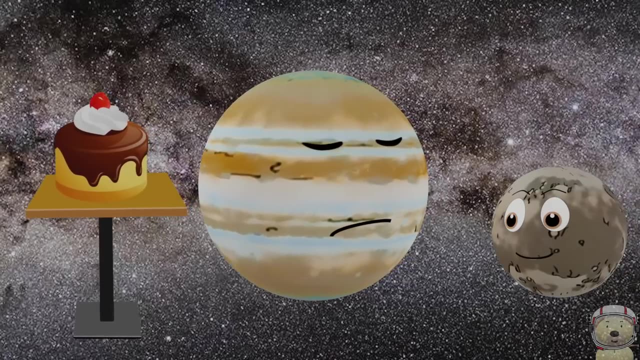 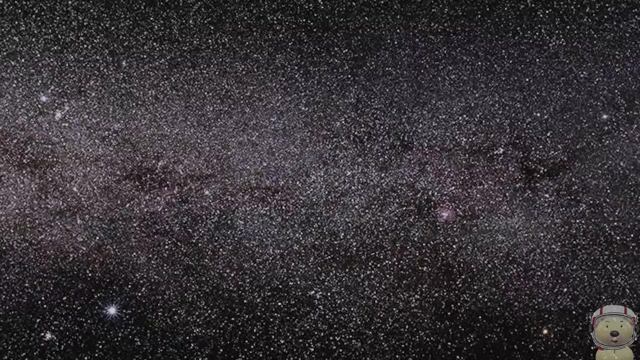 Hmm, Just imagine how big a moon would be if it was half the size of me, Half the size of Jupiter. Hmm, Lovely, Really lovely. Uh, I'm not sharing. My moons are called Charon, Nix, Hydra, Kerberos and Styx. 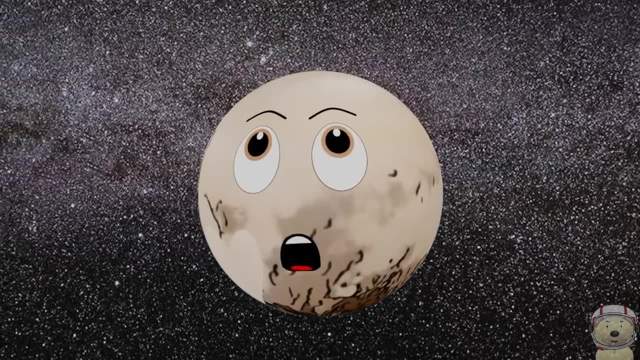 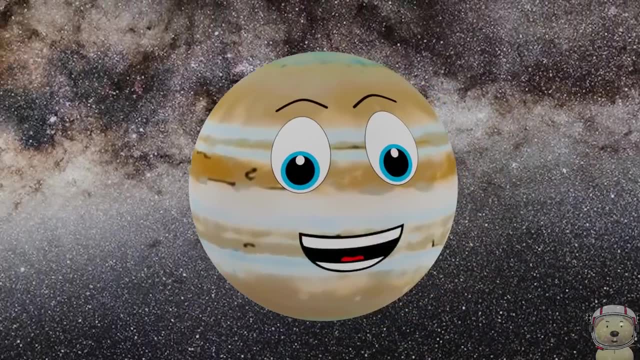 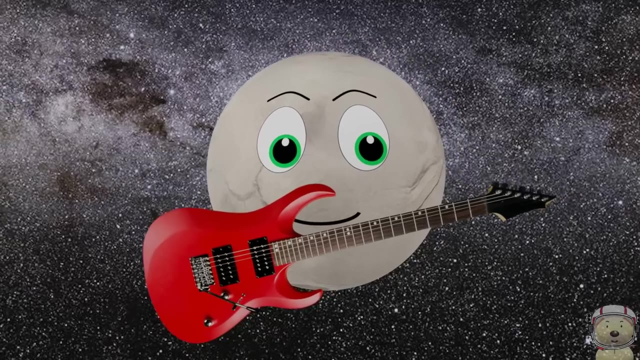 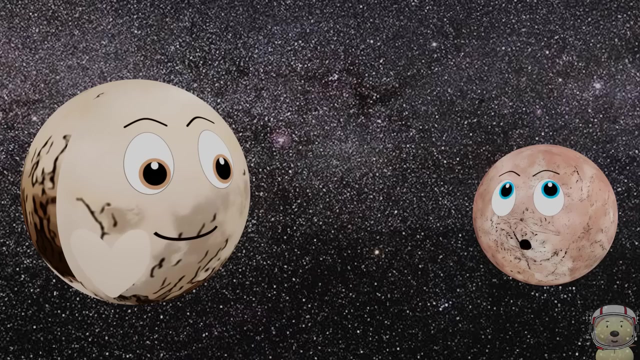 You're making these names up. No, I'm not. Charon, Nix, Hydra, Kerberos and Styx sounds like the names of people in a cool rock band: Macky Macky. how about you? Well, Pluto, I have one moon. It is nicknamed MK2.. 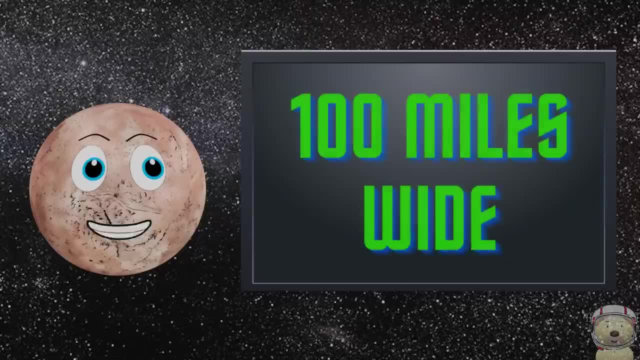 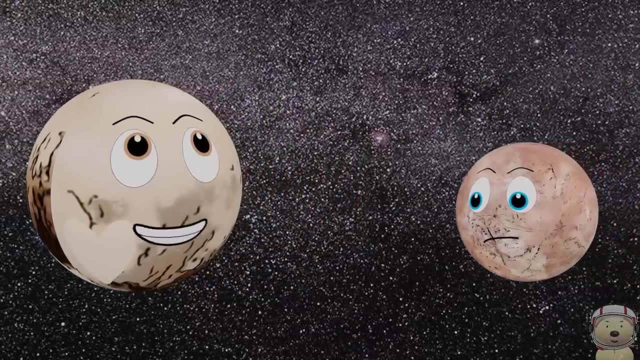 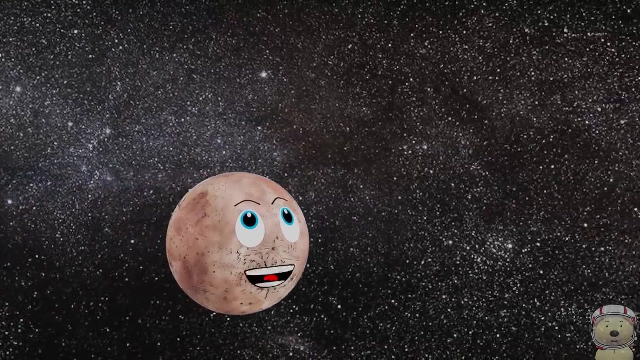 It isn't very big, as it is only about 100 miles wide, But it is my moon. Wow, That is a small but cool moon, Macky Macky, As I only have one moon, that makes me the most like planet Earth. 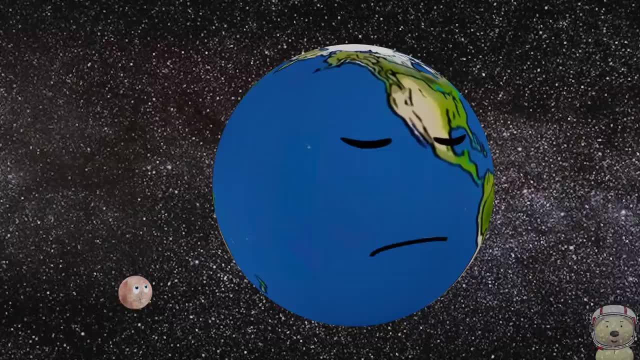 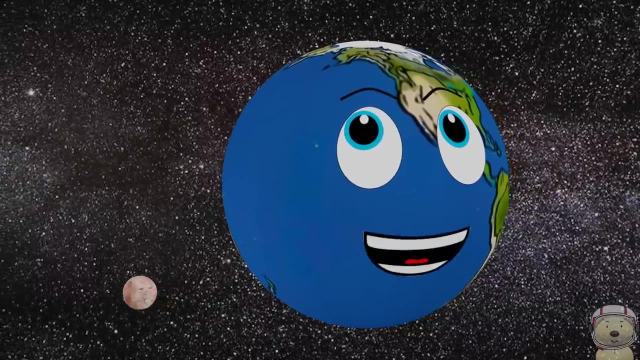 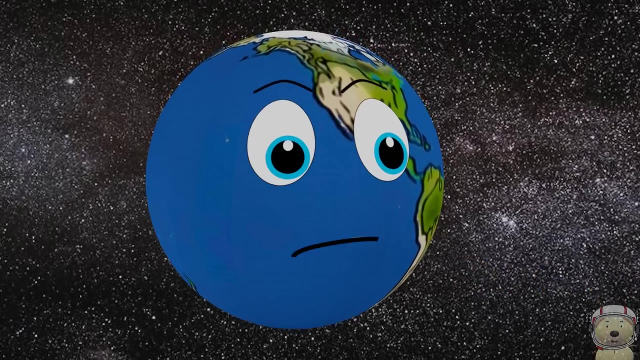 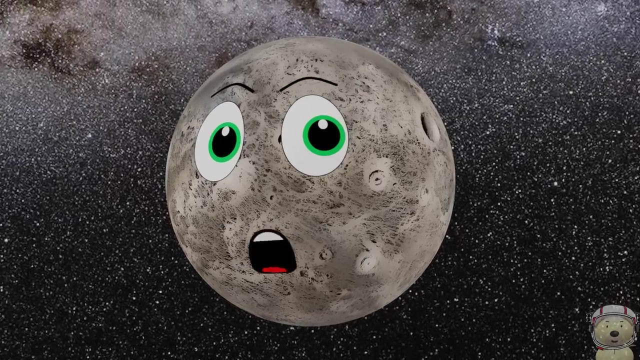 Hey Earth, we could be twins. Uh, We are so much alike I think you're confusing me with someone else. Macky, Macky, Come on brother. No Ceres, how about you? Well, actually, I don't have any moons. 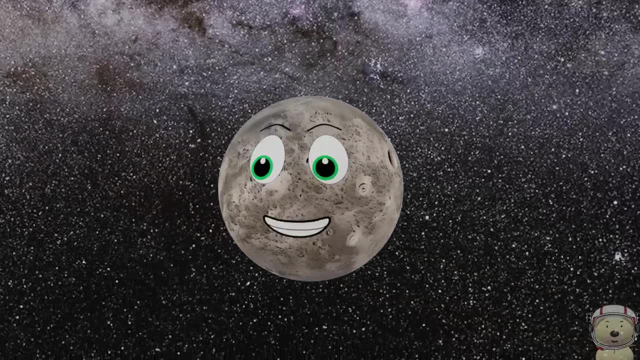 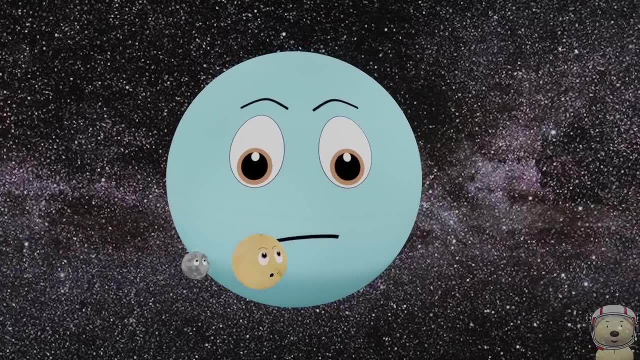 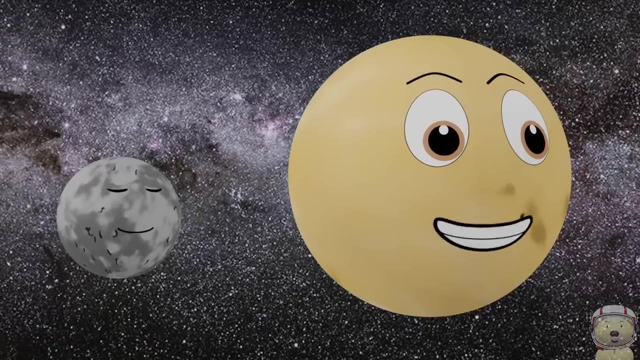 I am the only main dwarf planet in the solar system with no moon. That makes me so sad. Make some room please. Hey, Ceres, Come with Mercury and me. You can be in the No Moons Club. The No Moons Club. 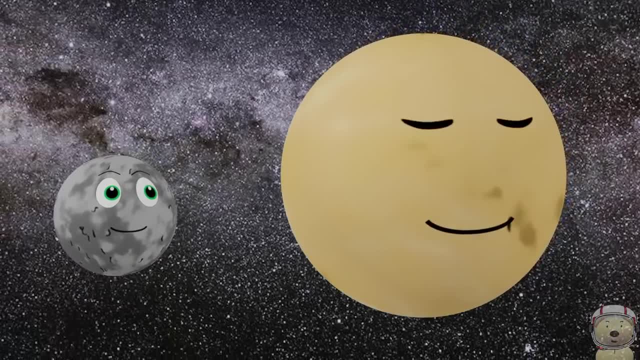 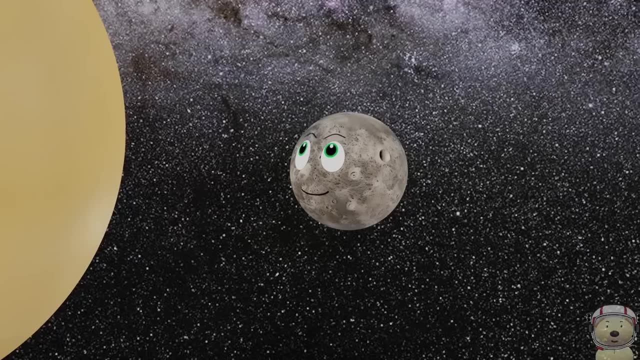 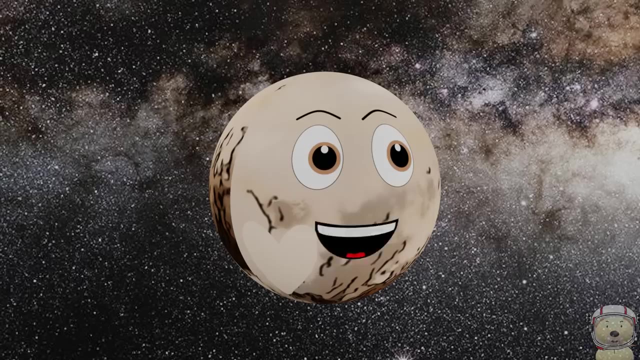 It's like the: We Have Lots of Moons Club. Well, it's way cooler. Hey, Alright, I'm cool. How much more awesome are we talking? Oh, so awesome, Huh, Maya. Yeah, Yeah, Yeah. 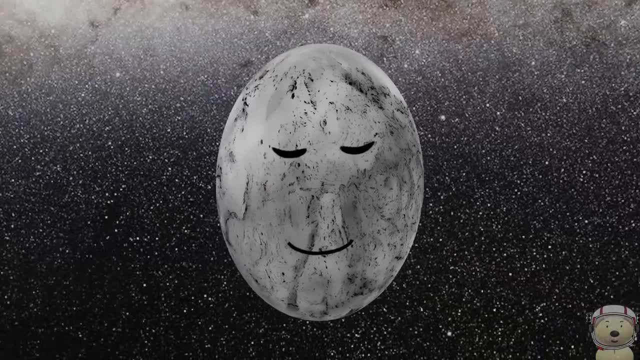 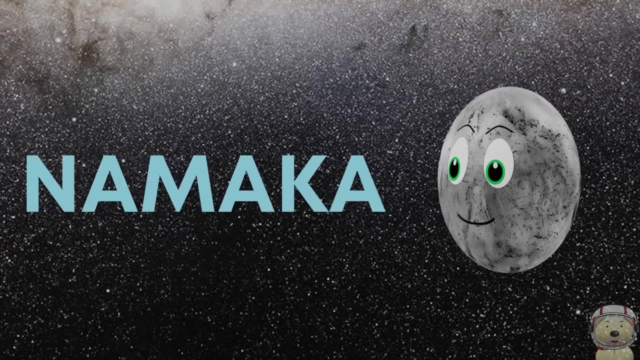 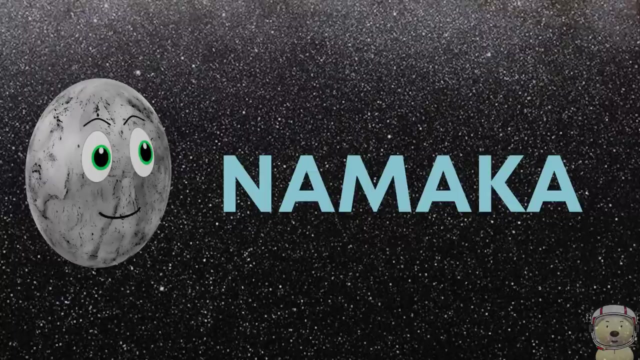 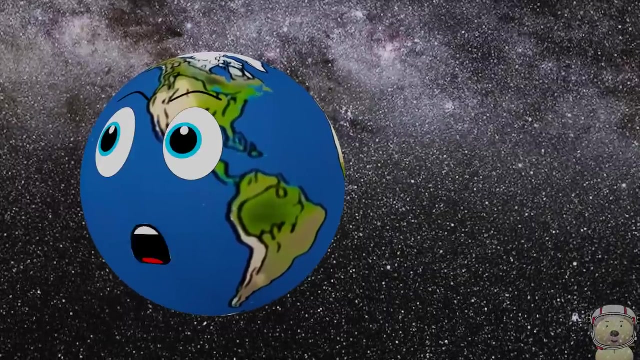 It's your turn. I have two moons. They are called Fried and Boiled Namaka and Hiyaka. Hiyaka is the goddess of the island of Hawaii. Namaka is a water spirit in Hawaiian mythology. It would be good one day if we could egg-splore your moon, Tamea. 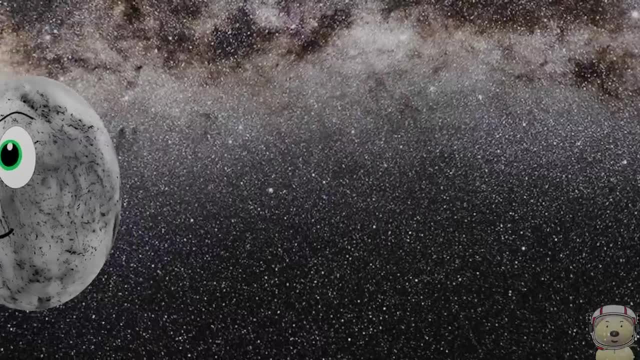 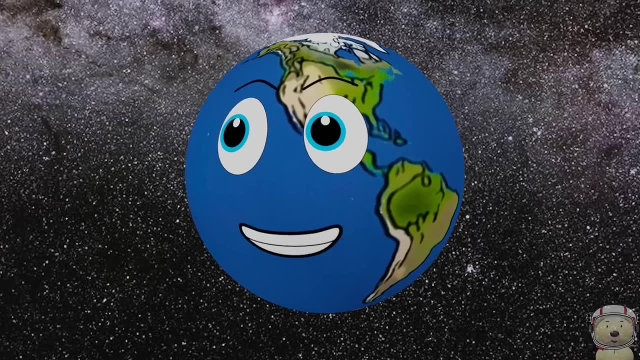 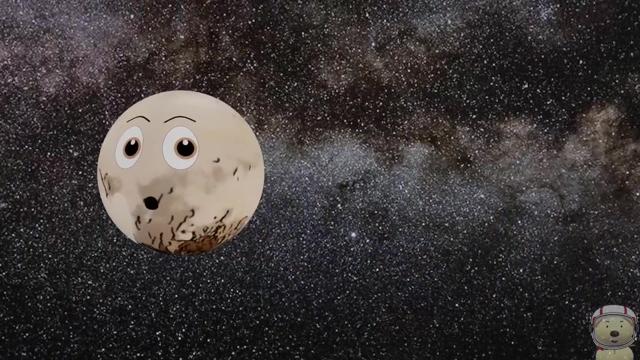 No, not doing this. He's made a quick egg-sit. No, I'm not an egg. Ha ha, ha, ha ha. Eris, how about you? Do you have any moons? Yes, Pluto, I certainly do. 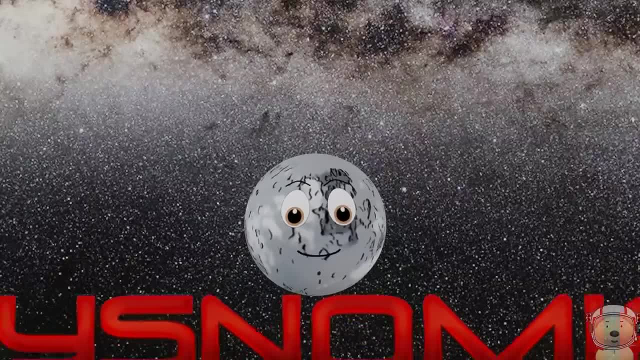 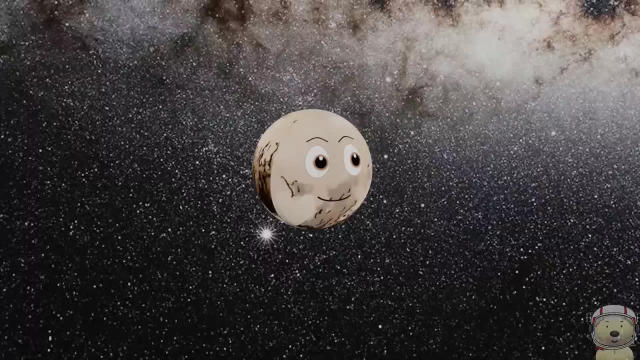 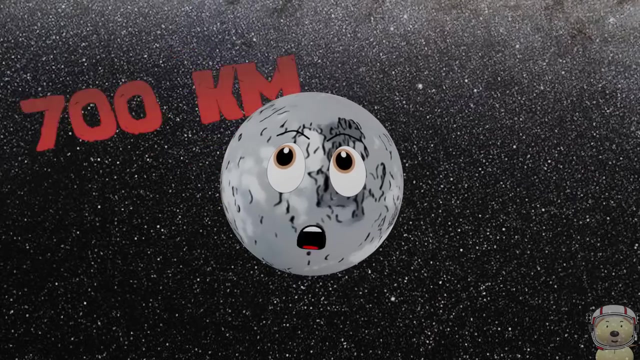 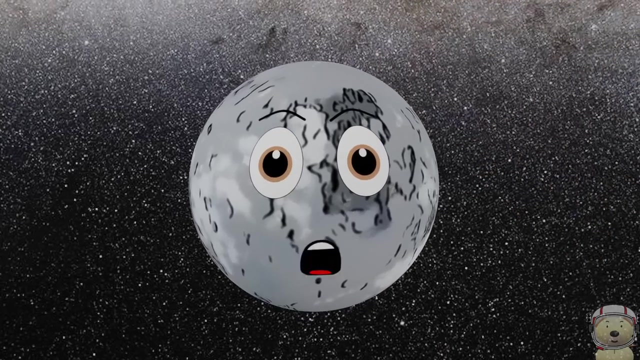 I have one known moon. It is called Dysnomia and is the second largest moon of a dwarf planet after Charon. That's great, Eris. How big is your moon? Probably about 700 kilometers. My moon and I are 68 times further away from the Sun than the Earth is.